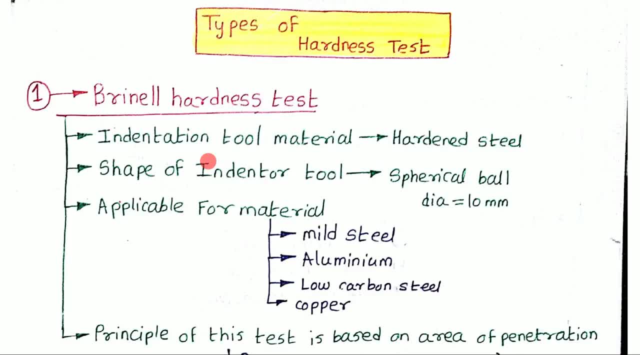 Hello everyone. let's understand the different kinds of hardness test. This topic is very important for vivas and interviews. They can ask what are the different kinds of indenter tools, which kind of hardness test is applicable for which kind of material? Such types of questions can be asked. 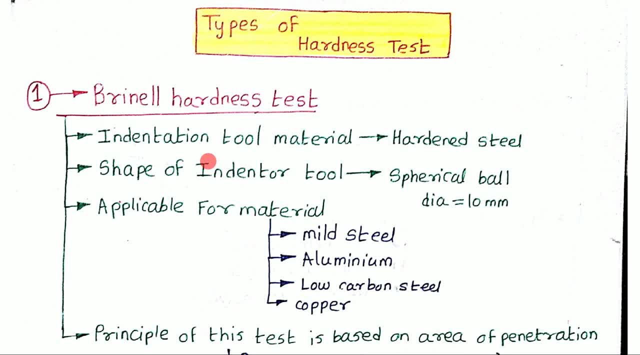 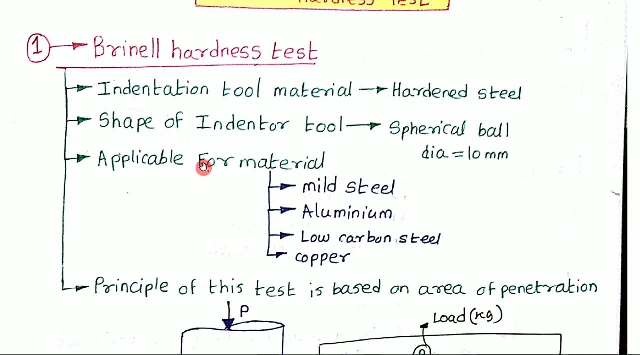 The first hardness test, the Brinell hardness test. Here the indenter tool is a spherical ball of diameter 10 mm. It is made up of hardened steel material. This Brinell hardness test is applicable for comparatively softer materials like mild steel, aluminum, low carbon steel or copper. 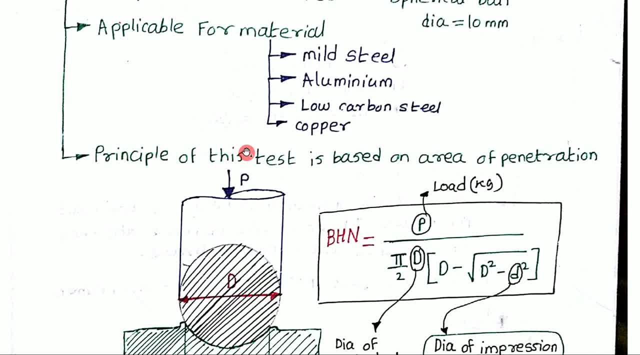 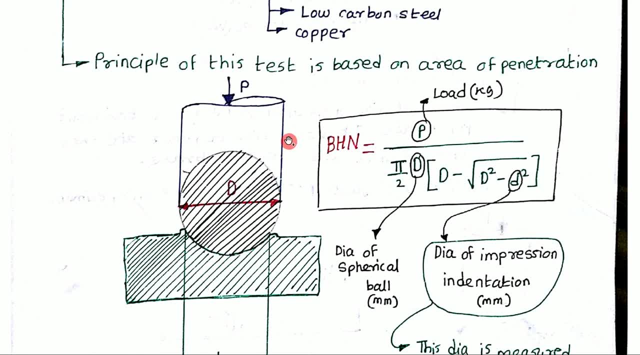 Here. the principle of this test is based on the area of penetration. This is the indenter tool and this spherical ball is the indenter of diameter: 10 mm. This indenter tool is pressed against this specimen with a load P. Due to this pressing action, the indenter penetrates into the ball. 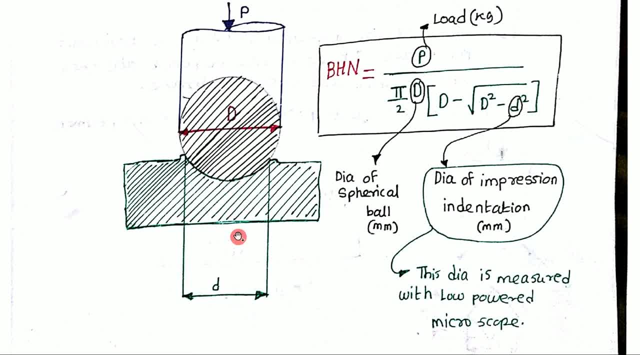 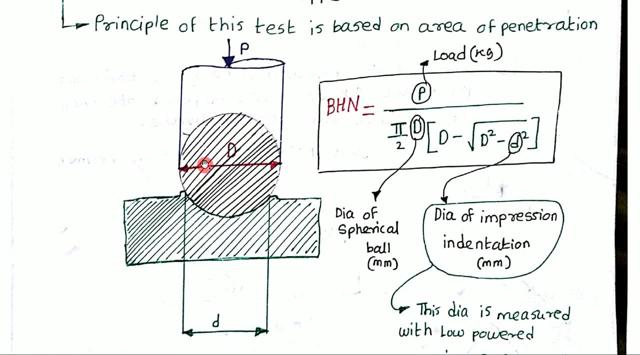 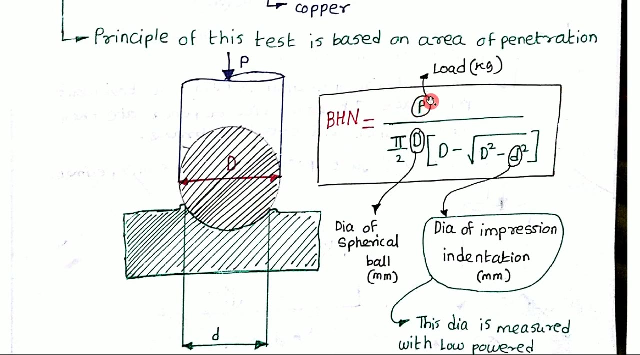 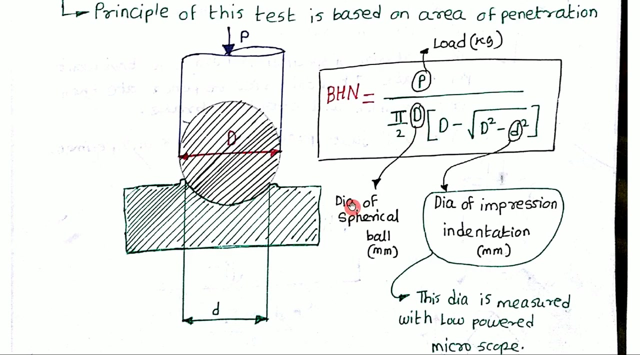 Here you can see that the Brinell hardness test is expressed as a typical well of 5,025 times higher than our normal silence test in village in a city where vaak capital, D is the diameter of the spherical ball, that is 10 mm. this small d is the diameter. 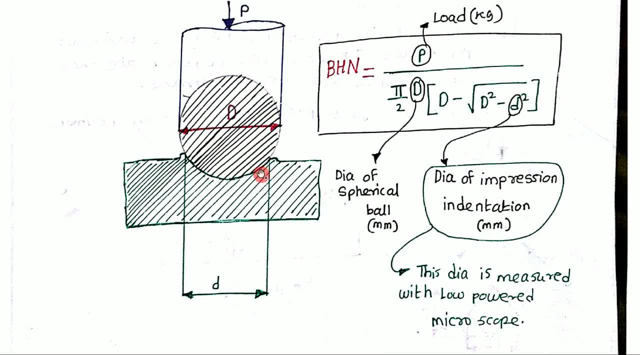 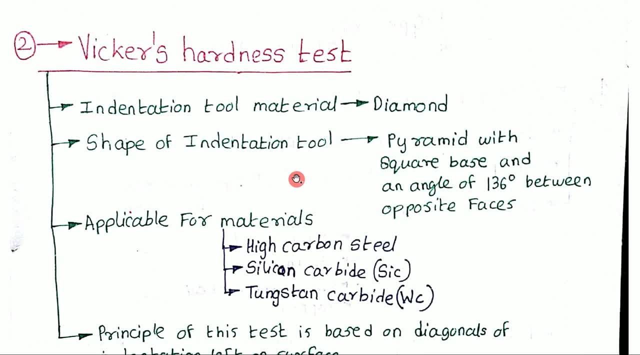 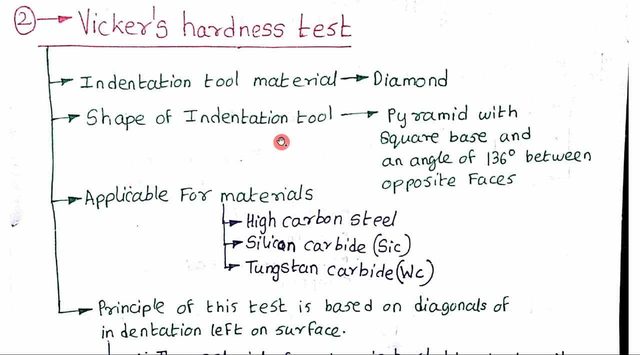 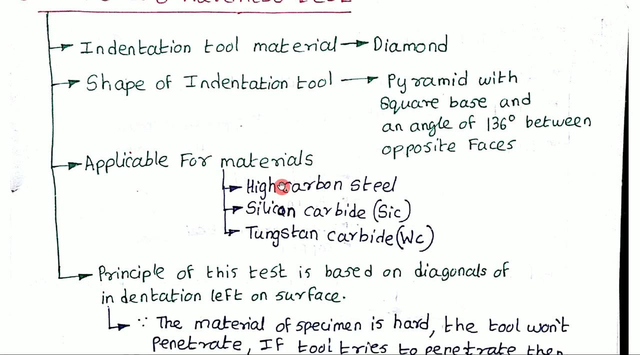 of indentation measured with the help of low powered microscope. The next hardness test is Vickers hardness test. here the indentation tool is of pyramid shape and the pyramid has a base square and the angle between the opposite faces of the pyramid is 136 degree. this is very important for viva's. they can ask this in viva. 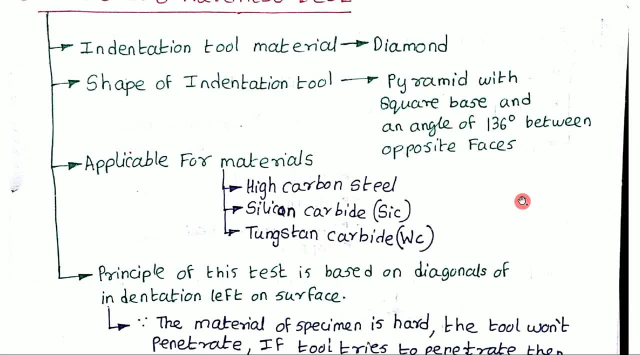 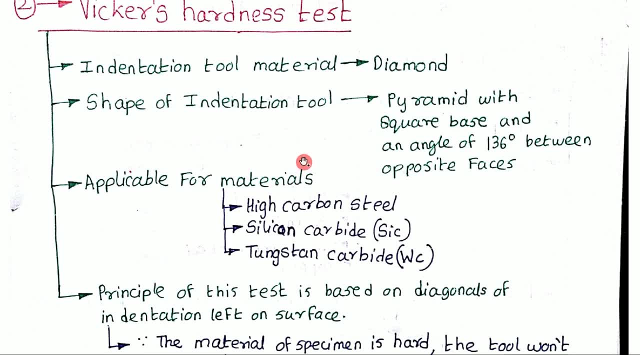 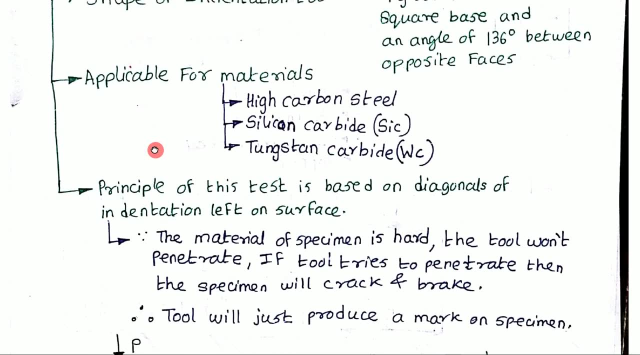 The material of the pyramid is diamond, see. this hardness test is applicable for diamond or harder materials like high carbon steel, silicon carbide, tungsten carbide. In this test, the indenter is not penetrating into the material, it is just producing a. 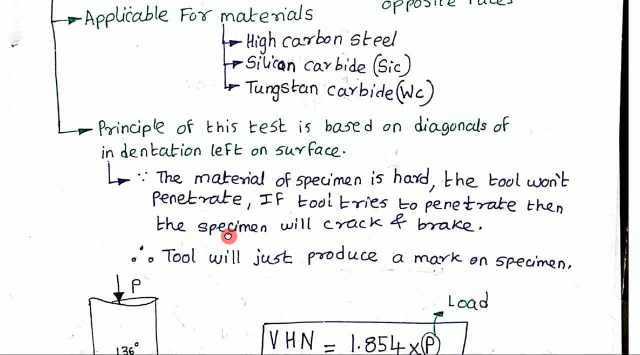 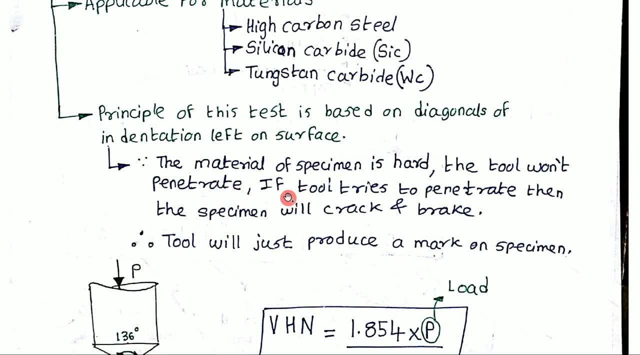 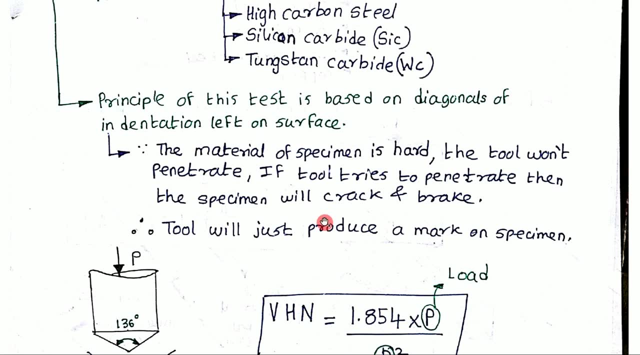 mark over the specimen. see what will happen if the tool tries to penetrate into the specimen, the specimen being hard in nature, it will break or it will crack. So this is the hardness test. So, therefore, the tool is just producing a mark on the specimen. the tool looks something. 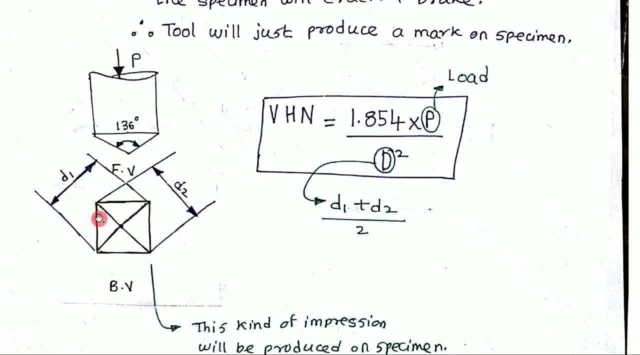 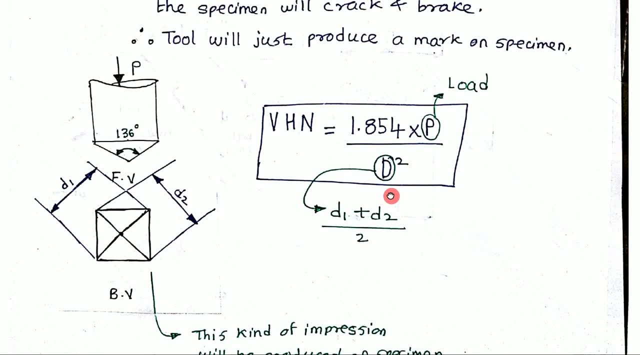 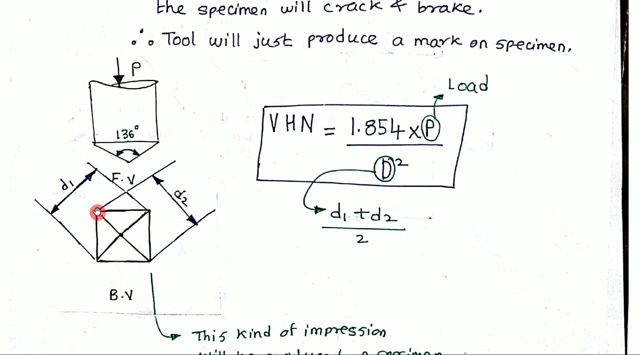 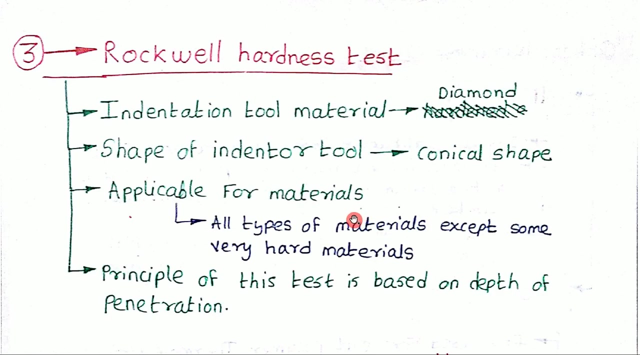 like this and it will produce a mark, something like this, on the specimen, and the VHN is given by this formula: this D2 is the diagonal, this D1 is this diagonal. The next hardness test is rockwell hardness test, here the shape of the indenter tool. 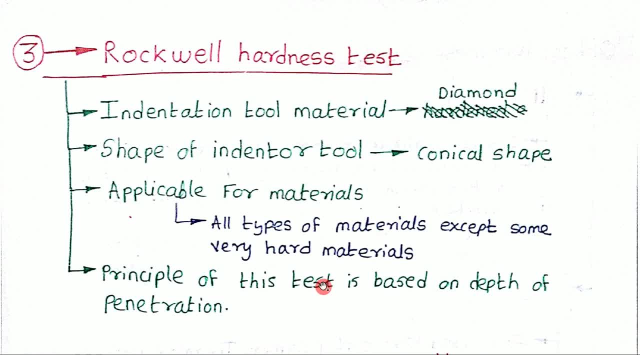 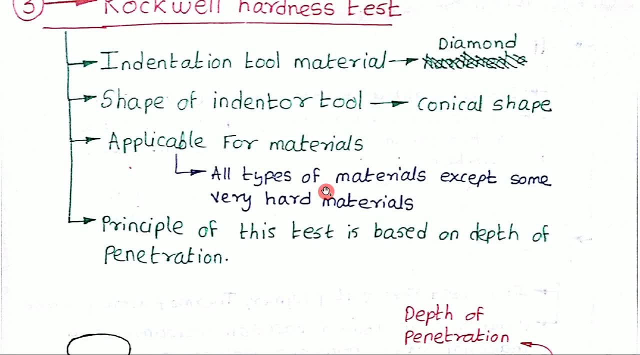 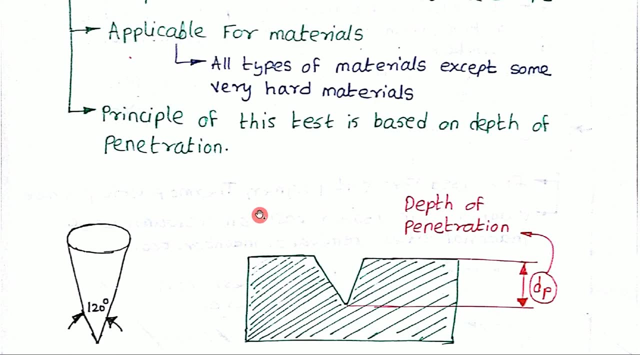 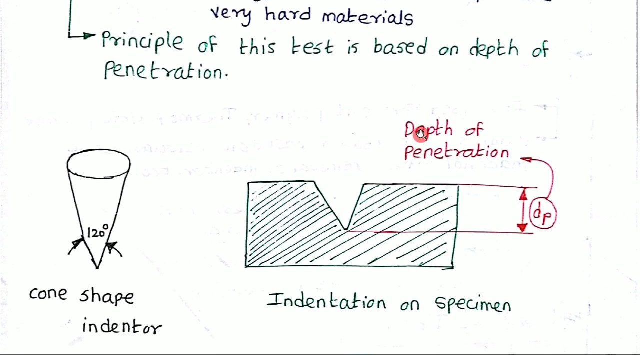 is conical and the material of the indenter tool is diamond. it is applicable for almost all kinds of material: 2. 3. very hard materials. the principle of this kind of test is based on the depth of penetration. depth of penetration: the Rockwell hardness number is inversely. 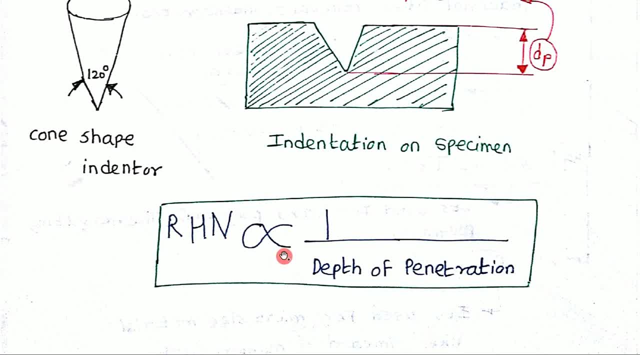 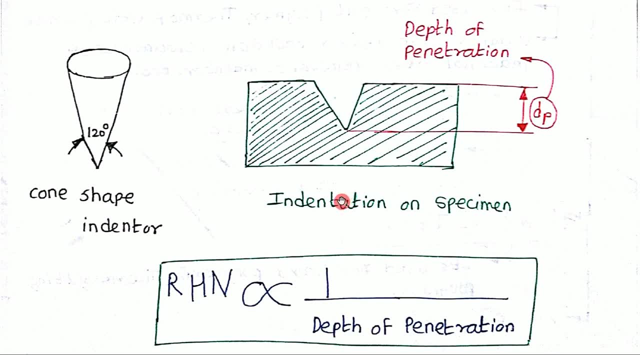 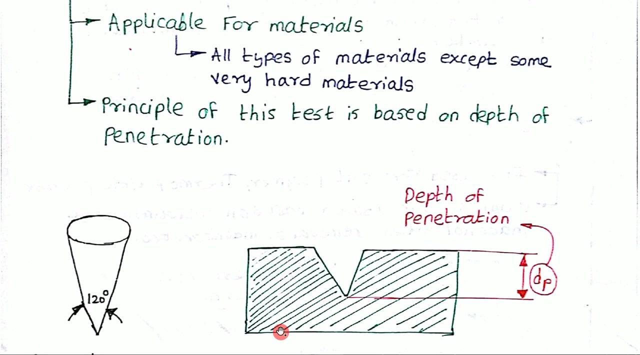 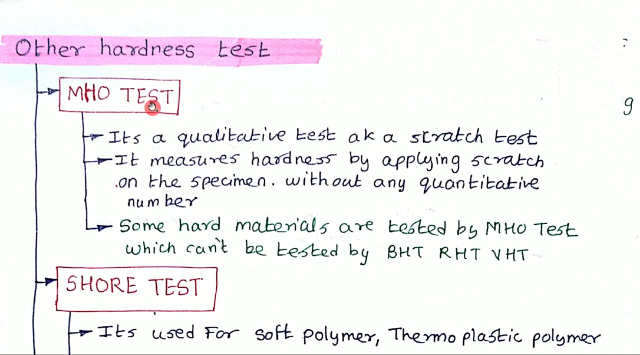 proportional to the depth of penetration. if the indent penetrates deeper in the material, the Rockwell hardness number is less. if the indenter able to penetrate deeper in the material, the Rockwell hardness number is high. similarly, there are some other kinds of hardness tests also, like MHO test. it is a quality test.